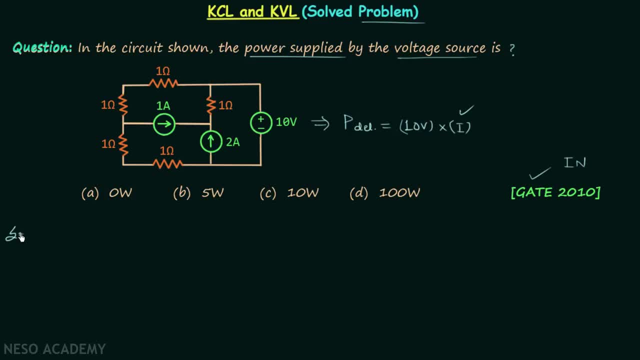 2010 exam. so let's move on to the solution and to begin with, i will first copy the given circuit and if you are making the nodes, then don't try to make the assumptions using the same circuit given in the question. this means, whenever you try to make the nodes, then always redraw the circuit while 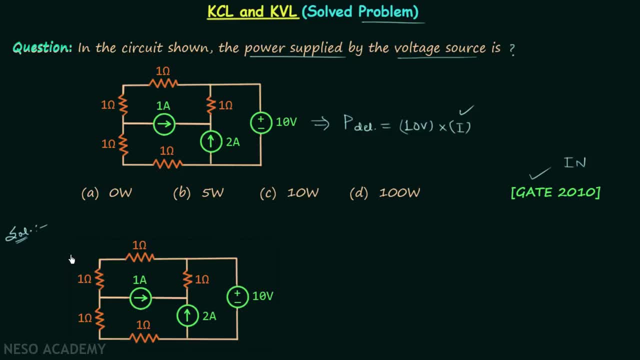 having the solution and we redraw the circuit to draw some assumptions and simplifications in the circuit. so don't make changes in the question, make changes in the circuit which you make changes without trying to finish the problem first. do the same in the second step, redraw in the solution. so let's move on to the first step and in the first step, 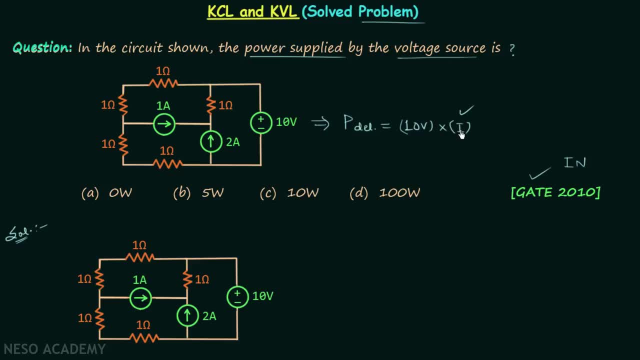 we will assign the direction to the current. I current, I will have this direction. it will leave the positive terminal and it will enter the negative terminal. why? because power is getting delivered and when power is delivered, the current leaves the positive terminal and enters the negative terminal. we 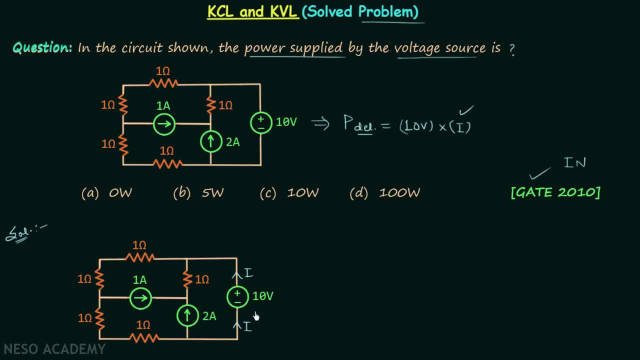 already know this point. now we will focus on the other two sources present in the circuit, and they are current sources. the first source here is providing the current equal to 1 ampere and this source here is providing the current equal to 2 ampere, and if you focus on this node then you will find 1. 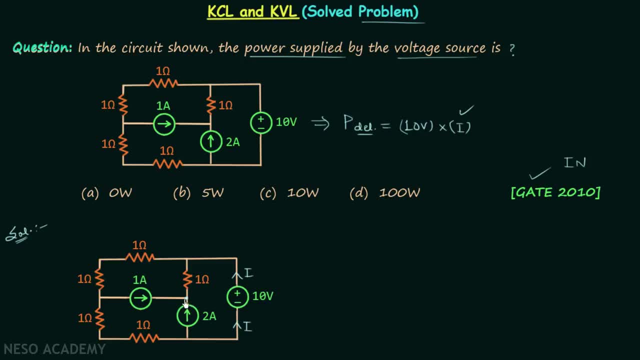 2 & 3 elements are connected to each other at this node. therefore this node is the principal node and we know at principal node current division will take place and therefore we will use KCL to find out current in this branch. 1 ampere current is entering the node 2 ampere. 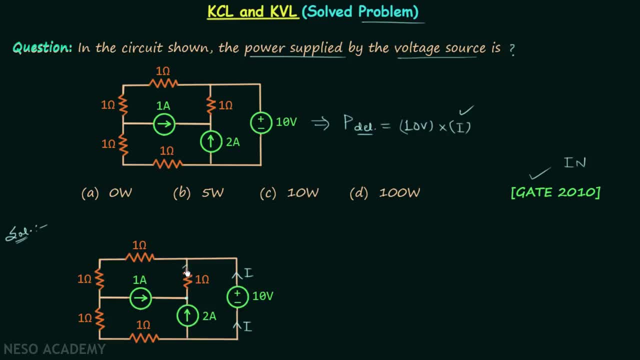 current is also entering the node and, let's say, current in this branch is in this direction. therefore, this current is leaving the node and we know, according to KCL, sum of entering currents will be equal to the sum of leaving currents and there is only one leaving current, so sum of these two currents will be equal to. 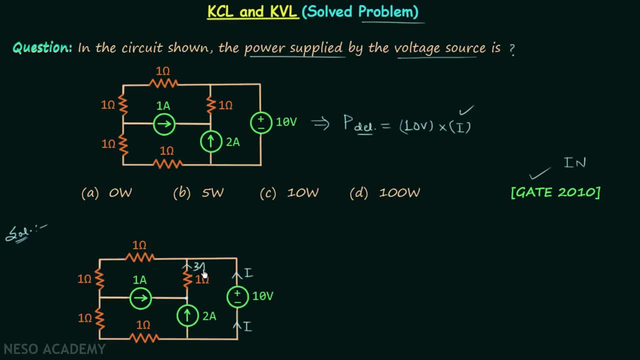 this current. so 1 ampere plus 2 ampere is equal to 3 ampere, and from here we are getting current I. so at this node we again have current division, because 1, 2 and 3 elements are connected here. so this is a principal node. 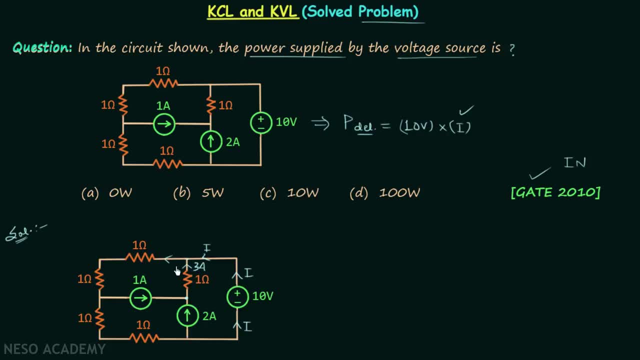 and according to KCL, this current, which is the leaving current, will be equal to 3 ampere plus I, because these two are the entering currents. so we have I plus 3 current in this branche. this node here is the simple node. two elements are: 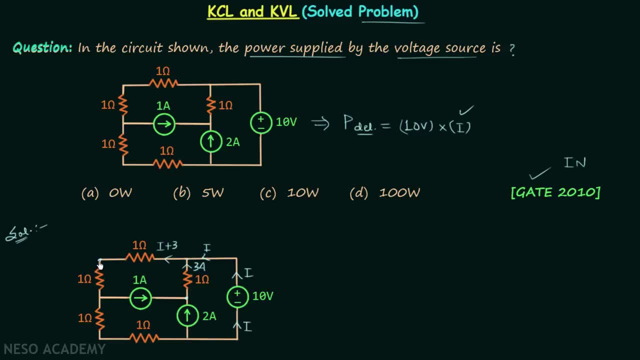 connected here. therefore, this is the simple node, and at simple node no current division takes place. therefore, same current I plus 3 and so on take place. the node are connected to. there is no current division takes place, then in that simple node is supportedので. Law plus yard chi n stinks straight. so much, learners do not be. a means constitutes bad. 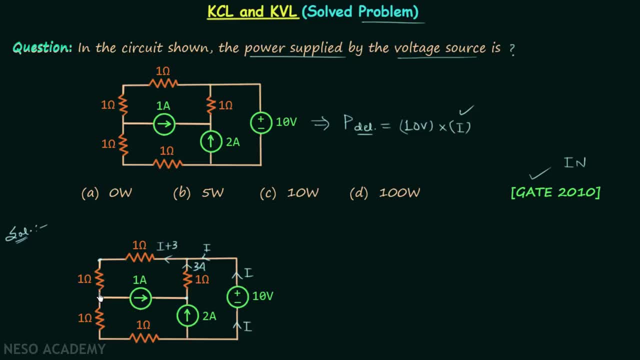 even if you speak English, also from French, which I would be worried. I can't find English at all and therefore please don't ask questions. fees will flow through this resistor as well. so here we will have I plus 3 current, and this current I plus 3 is entering the node and 1 ampere current is leaving. 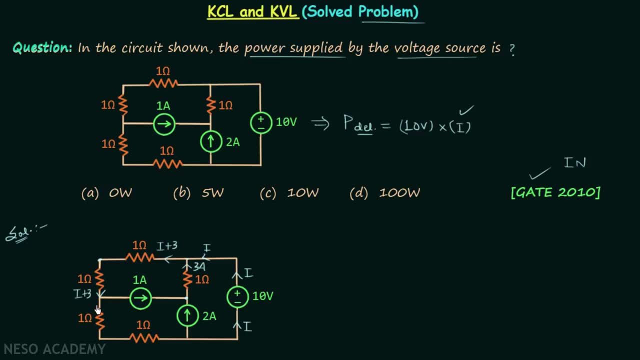 the node, let's say current in this branch, is having this direction. so this current will be equal to I plus 2. you can apply KCL or you can simply look at the fact that I plus 3 is the current entering, out of which 1 ampere current is. 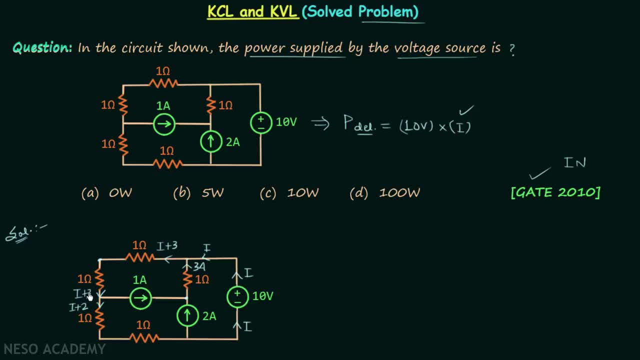 leaving. this means I plus 3 is now reduced to I plus 2. 1 ampere current is moving in this branch, moving forward. we again have the simple node and at simple node no current division takes place. so I plus 2 will be the current through. 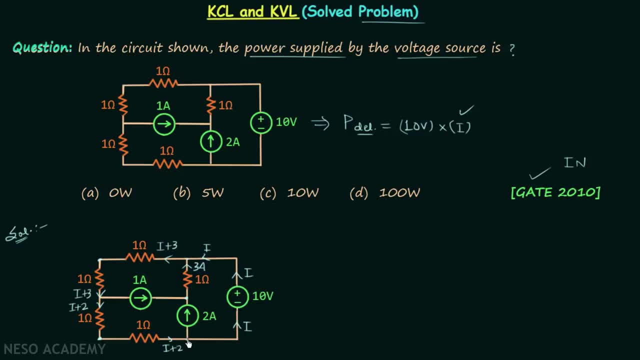 this resistor as well. now, at this node, current division will take place because, like this node, this node is also a principal node and therefore we will apply KCL. or we can think in a very simple manner that I plus 2 is the current entering, out of which 2 ampere current is the 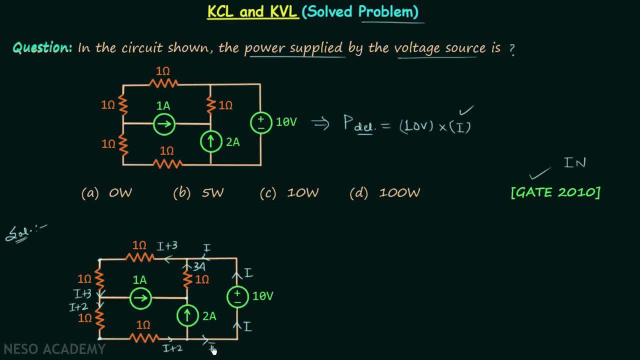 leaving. so here we will have I current left, which is true now. after this, we have currents in different branches and now we can apply KVL. and to apply KVL, we will choose the outer loop. I am selecting the outer loop because if you select any other loop, you have to include one or two current. 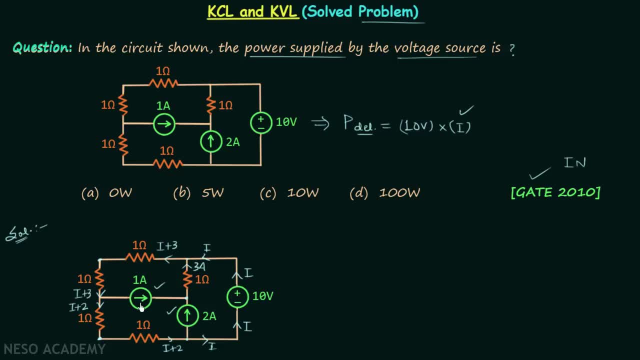 sources and we don't know about the voltage across these two sources. therefore, we will try not to include them and hence we will select the outer loop. so let's quickly apply KVL. we will start from this point, moving in this direction, in the direction of current I. we have one source providing. 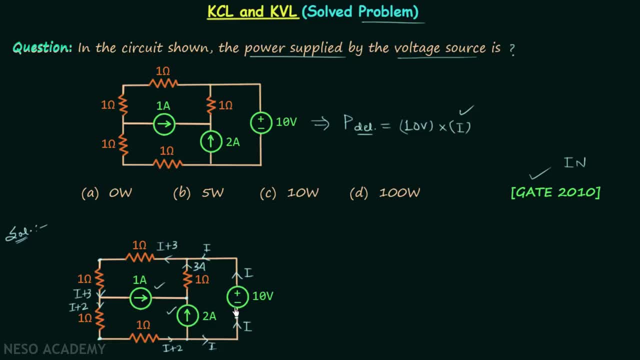 10 volts as the voltage and you can see that the potential is rising. therefore we will take the positive sign. so we have plus 10 volts. then we have one resistor and we know resistor in the same direction of the current will give us the drop in potential. therefore we will have the negative sign and the 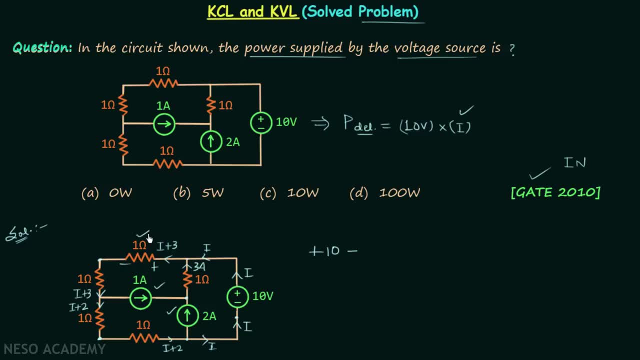 voltage drop will be equal to the resistance multiplied to the current, so 1 x 2, I plus 3, which will give us I plus 3. now moving forward, we have one more resistance having the value 1 Ohm, through which I plus 3- current is. 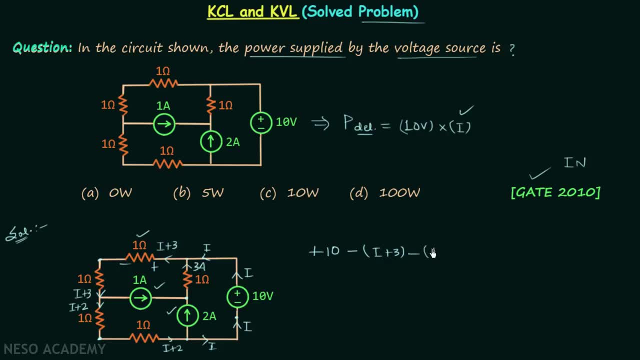 flowing, and therefore we will have minus I plus 3. similarly, for this resistor, we have minus I plus 2, and for this register, we have minus i plus 2, and then we move back to the same point. therefore, we will equate this with 0.. now, when you simplify this, you will get 10 minus 10 minus 4 times. 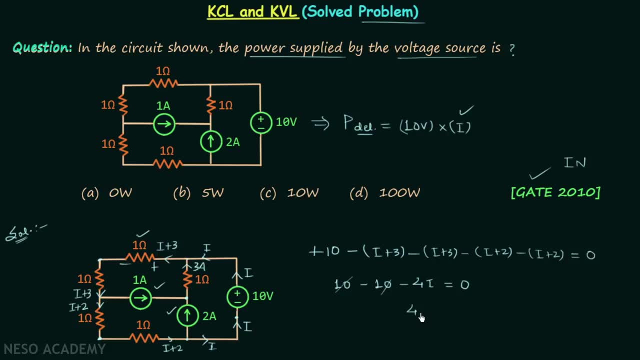 i equal to 0.. 10 and 10 will cancel, so we have 4 times i equal to 0, which implies current i is equal to 0 and now it is very clear that power delivered by this source will be equal to 10 volts.